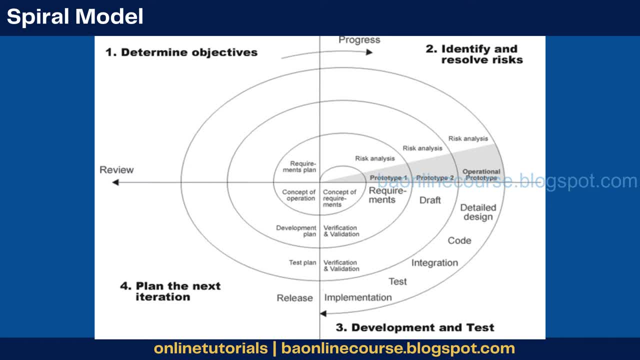 give you a context of where this could be useful and then I think you will be able to relate. Now let's say there is a new technology, a completely new technology, and you know you want to implement your core system in that particular technology, So existing system. 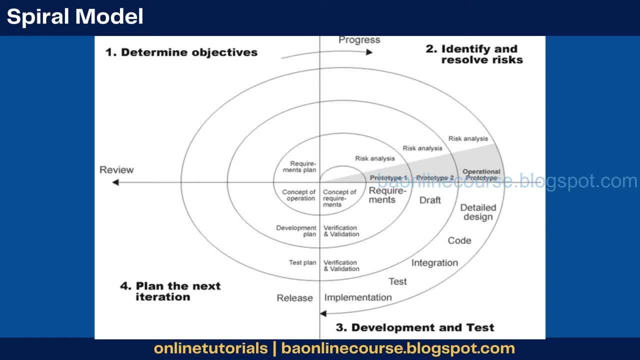 is, let's say, mainframe system, an old green screen system wherein you don't even have a GUI and all is you will have to type in using your keyboard. So that kind of system is there, But it is your core system And you want to, you know, migrate that into a latest technology, Let's say Java, using 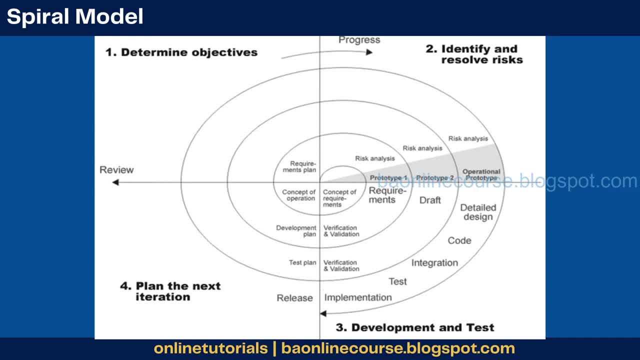 straps or whatever it is. Now you know there are too many unknowns in this project, So you could feel that you know whether that new technology, Java, could support the kind of volumes which are being processed by my system. So let's say that there are like you. 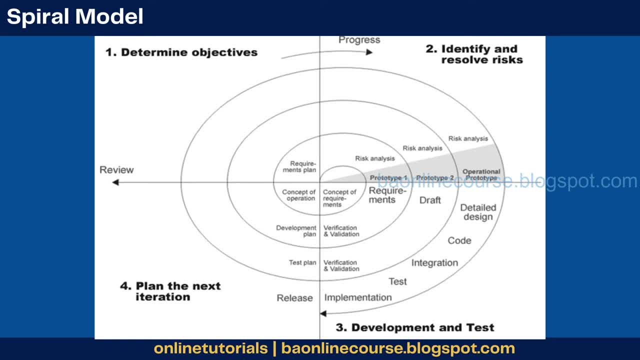 know 2000 transactions which are 2000 transactions which are being processed by my system. So let's say that there are, like you know, 2000 transactions which are 2000 transactions which are, or you know, 20 million transactions which have been processed in a particular 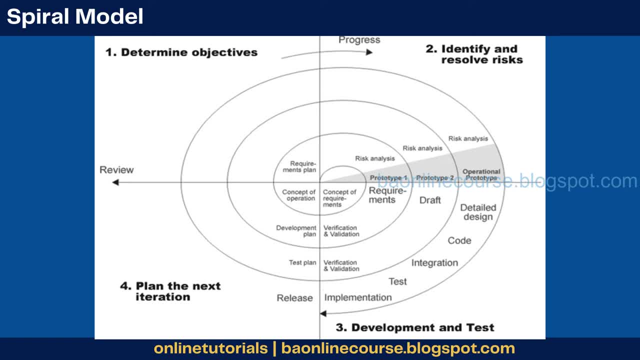 day. Ok, Now the old system is supporting, you know that, but you don't know whether the new system would support those kind of number of transactions or not. Ok, So you should not be in a situation that you capture all the detailed requirements about the system. 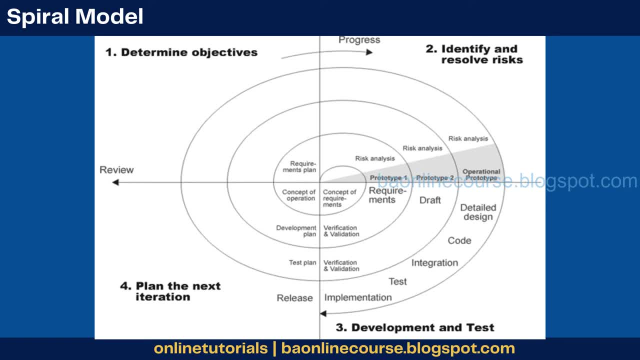 You spend like 6 months capturing all the detailed requirements. You spend some a million dollars for those requirements and then during the design you will figure out. you know what this system does not work and support the number of transactions. okay, Now all your money which you have spent. 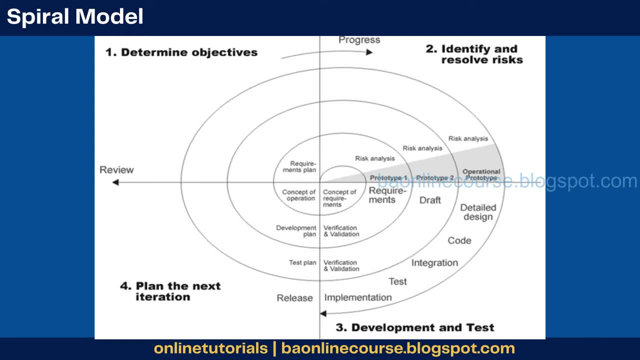 all the million dollars for capturing the detailed requirements is gone waste. So there is no use of it because you know you cannot implement in the new system right Now. at that point you would think you know we should have actually looked at this risk. 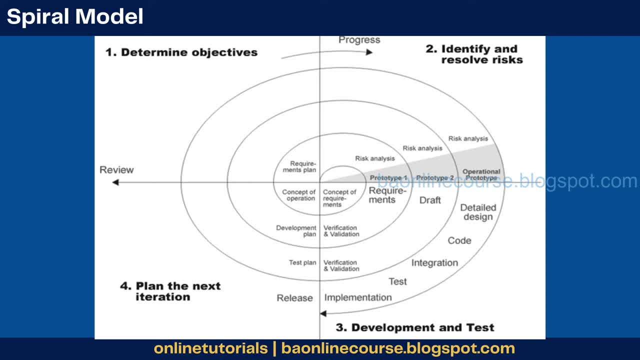 right at the start of the project, right? So that's exactly what we're doing in a spiral model. So when you start the project and then figure out there are too many layers, what you would do is you'll find out what are my key objectives of my system. 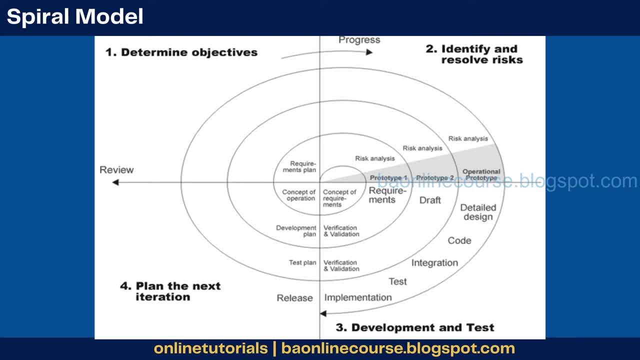 You'll find that first right. Let's say, my first key objective of the project is to support that volume of transactions Because, you know, not all technologies can support. So I just want to make sure that before I start the detailed implementation of the system. 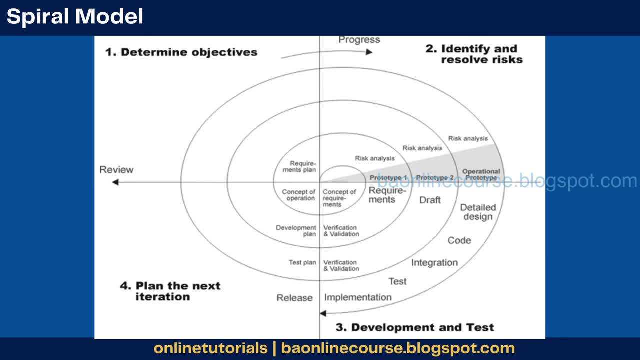 you know, I'll make sure that the technology is supported. So the first step is basically to figure out whether the number of transactions are supported or not. So I'll figure out, you know what are the risks involved in it, And then do some small. you know. 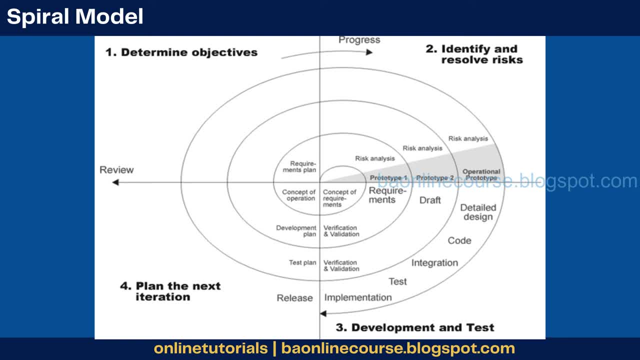 I'll pick up one functionality and then ensure that that 20 million transactions can be processed right. Once that is successful- only once that is successful- then I'll move on to the next topic, the next set of objectives, and then you know. 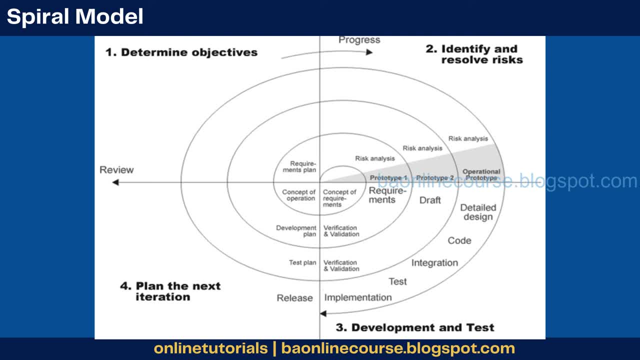 incrementally go with the development right. So says my system right. So my second objective could be: you know it should support some 100,000 customers, 100,000 users. When 100,000 users log in, the system should not crash. 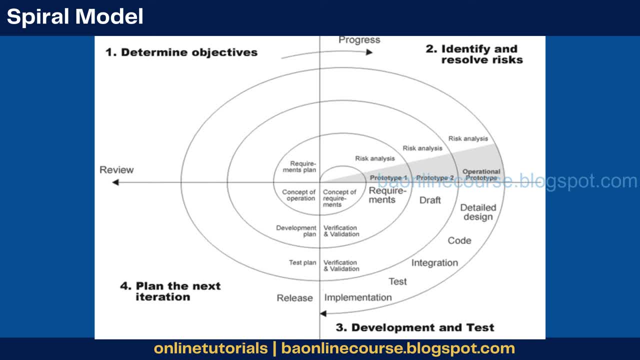 Then I'll go back and then do some development and make sure that you know it is So. the second objective is to ensure that number of users are supported And let's say you know you've done that development as well. 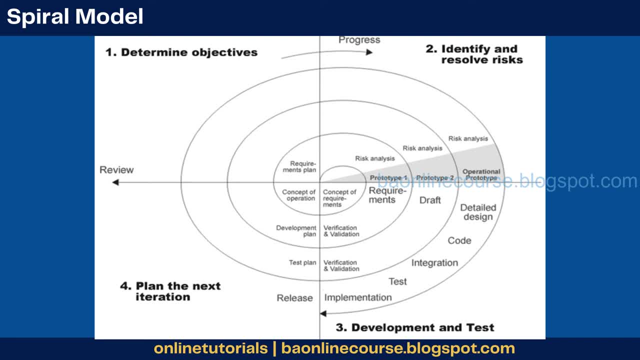 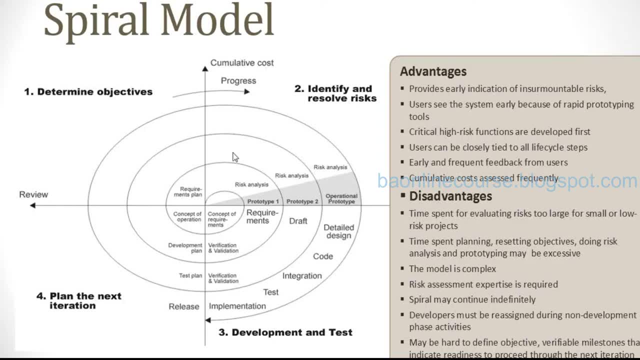 Now the third objective or key requirements would be: you know, I want these three new features to come in right, So you just do the development of that and then you know, incrementally or at risk-based approach, you're taking up. 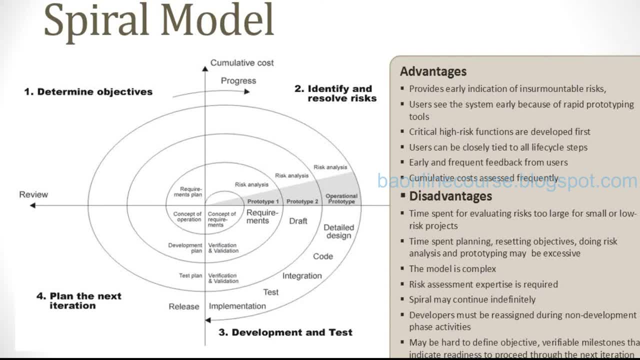 and with each prototype you're developing the system right. So this way you know at any point. if you feel that the risks are high and you know you're not able to meet the requirements, you could just stop the project. 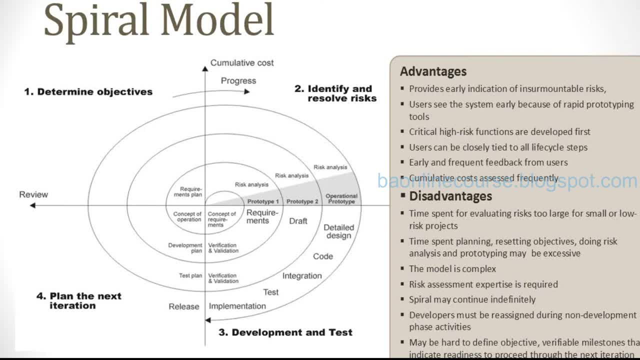 So your costs are much more, you know, contained in that kind of scenario. even if the project fails, you are not wasting a lot of money, okay, so that is basically a risk-based approach: where you are, you know, judiciously using your, your budgets, and then try trying to implement the system within the minimum.